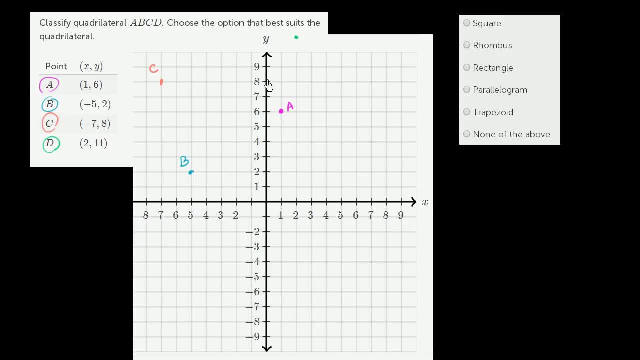 This is 10,. 11 would be right like this, So that would be two comma 11.. If we were to extend this, this is 10, and this is 11 right up here, two comma 11.. So let's see what this quadrilateral. 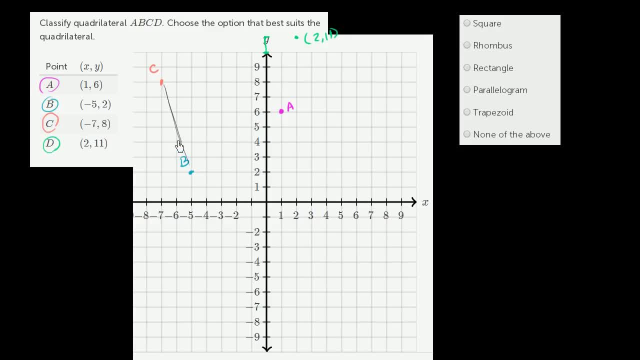 looks like You have this line right over here, this line right over there, that line right over there, and then you have this line, you have this line like this, like this, and then you have this like this. So, right off the bat, well, it's definitely a quadrilateral. 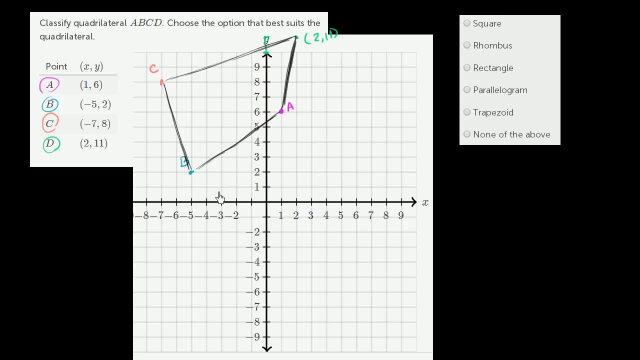 I have four sides, but the key question: are any of these sides parallel to any of the other sides? So just looking at it side, CB is clearly not parallel to AD. that you just can look at it Now. it also looks like CD is not parallel to BA. 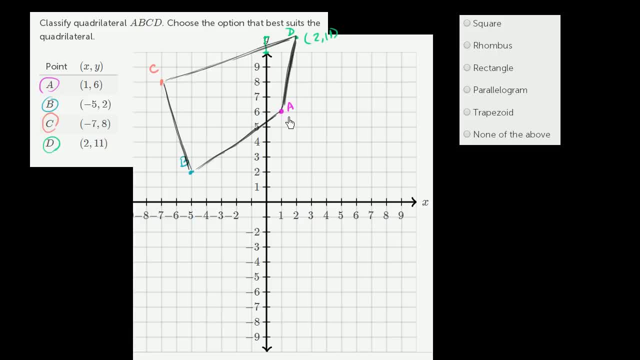 but maybe I just drew it badly. Maybe they actually are parallel, So let's see if we can verify that. So the way to tell whether two things are parallel is to actually figure out their slopes. So let's first figure out. let's figure out their slopes. 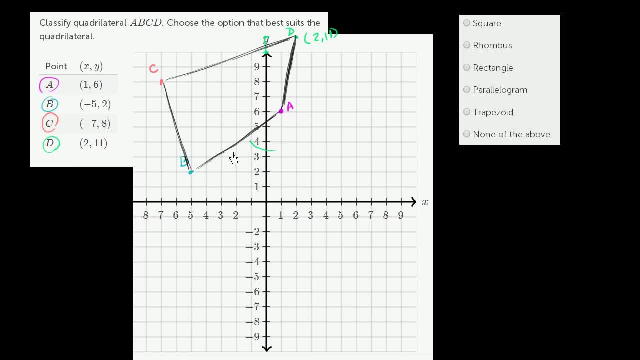 So let's first figure out their slopes. So let's first figure out their slopes. Let's figure out our slope of AB or BA. So let's figure out our slope. here, Your slope is going to be the change in Y over your change in X. 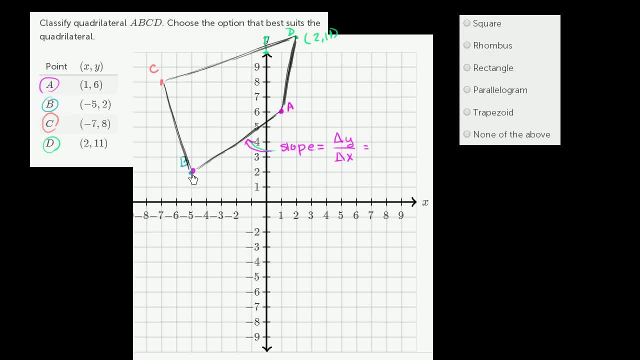 And in this case, you could think of it as we're starting at the point negative five comma two, and we're ending at the point one comma six. So what's our change in Y? Our change in Y? we go from two. we're going from two all the way to six. 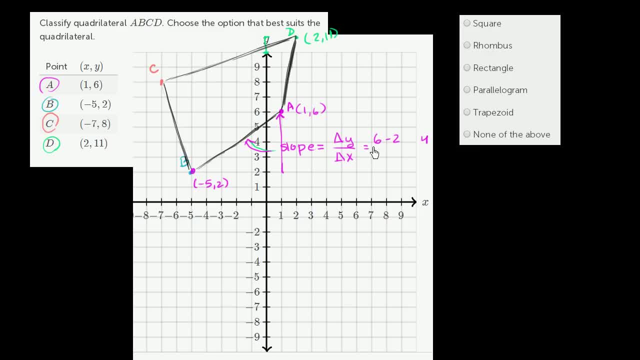 Or you could say it's six minus two. our change in Y is four. What's our change in X? Well, we go from negative five negative five to one. So we increased by six, Or another way of thinking about it, one minus negative five. well, that's going to be equal to six. 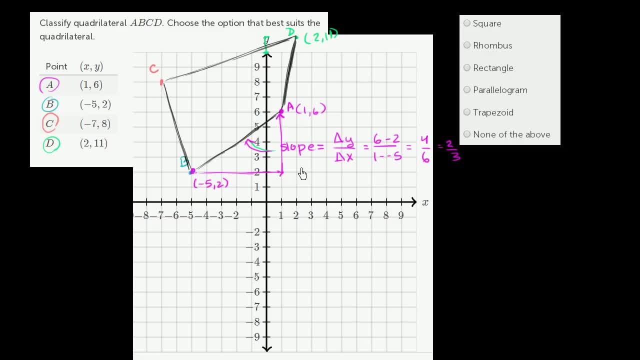 So our slope here is two thirds, It's two over three. Every time we move three in the X direction, we go up, go up two in the Y direction. Move three in the X direction, go up two in the Y direction. 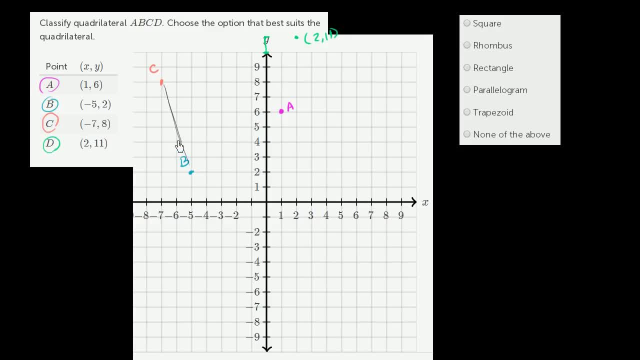 looks like You have this line right over here, this line right over there, that line right over there, and then you have this line, you have this line like this, like this, and then you have this like this. So, right off the bat, well, it's definitely a quadrilateral. 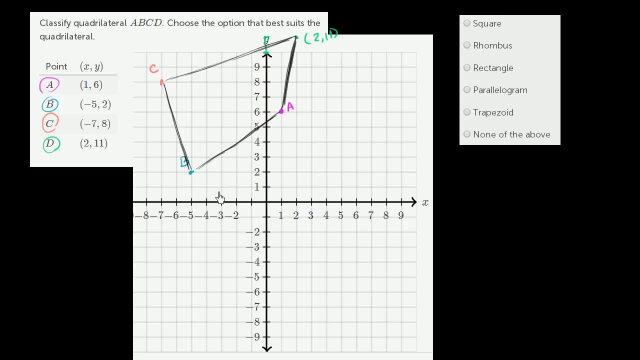 I have four sides, but the key question: are any of these sides parallel to any of the other sides? So just looking at it side, CB is clearly not parallel to AD. that you just can look at it Now. it also looks like CD is not parallel to BA. 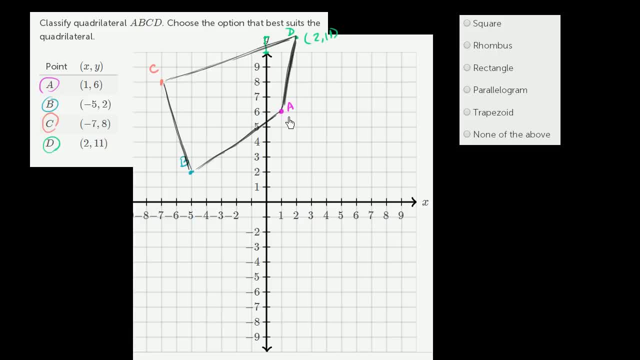 but maybe I just drew it badly. Maybe they actually are parallel, So let's see if we can verify that. So the way to tell whether two things are parallel is to actually figure out their slopes. So let's first figure out. let's figure out their slopes. 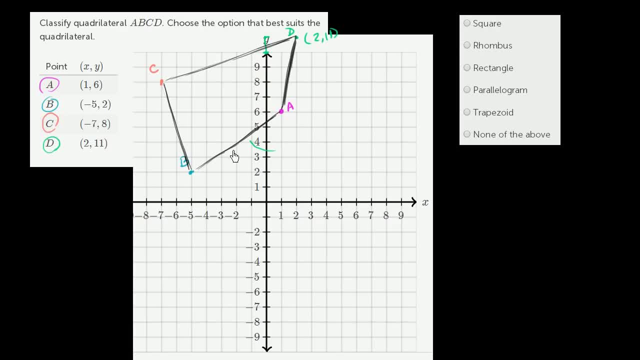 So let's first figure out their slopes. So let's first figure out their slopes. Let's figure out our slope of AB or BA. So let's figure out our slope. here, Your slope is going to be the change in Y over your change in X. 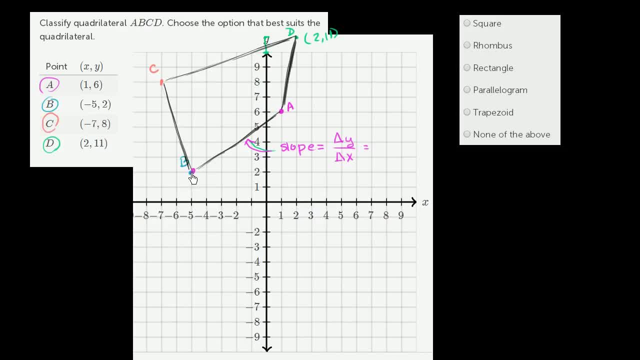 And in this case, you could think of it as we're starting at the point negative five comma two, and we're ending at the point one comma six. So what's our change in Y? Our change in Y, we're going from two all the way to six. 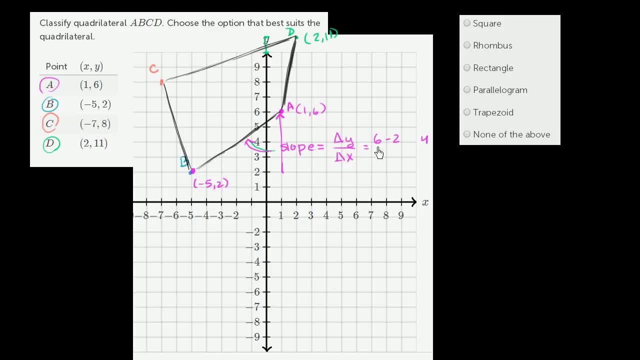 Or you could say it's six minus two. Our change in Y is four. What's our change in X? Well, we go from negative five to one. So we increased by six- Or another way of thinking about it- one minus negative five. 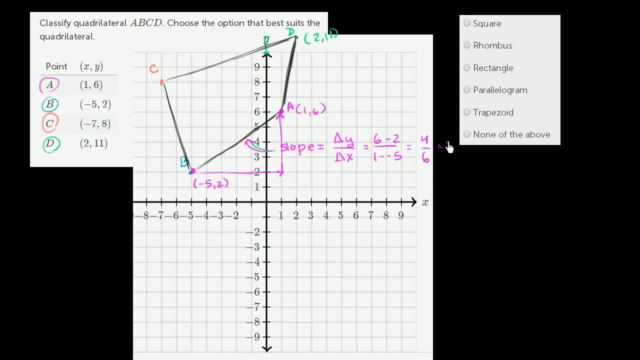 well, that's going to be equal to six. So our slope here is 2- 3rds. It's two over three. Every time we move three in the X direction, we go up two thirds, Up two in the Y direction. 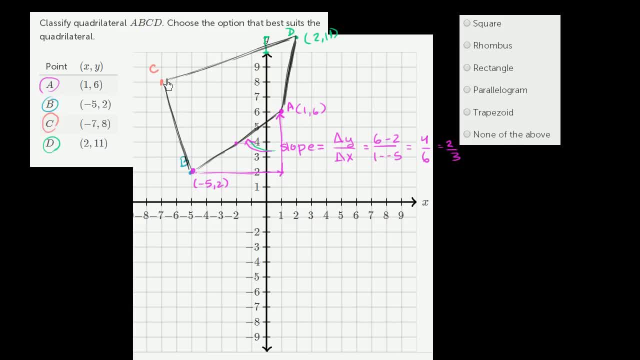 Move three in the X direction, go up two in the Y direction. Now let's think about line CD up here. Line CD, line CD. what is our slope? Our change in Y over change in X is going to be equal to. let's see. 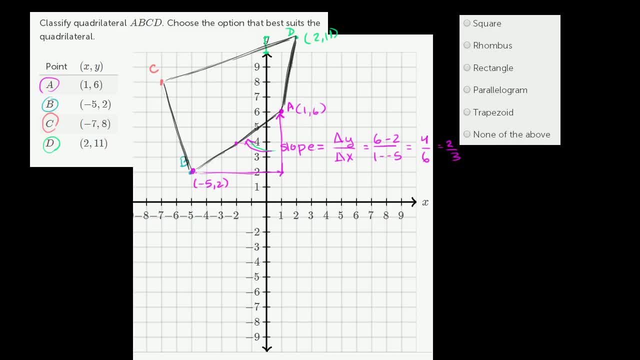 Now let's think about line CD up here. Line CD, line CD. what is our slope? Our change in Y over change in X is going to be equal to. let's see our change in. let's figure out our change in X first. 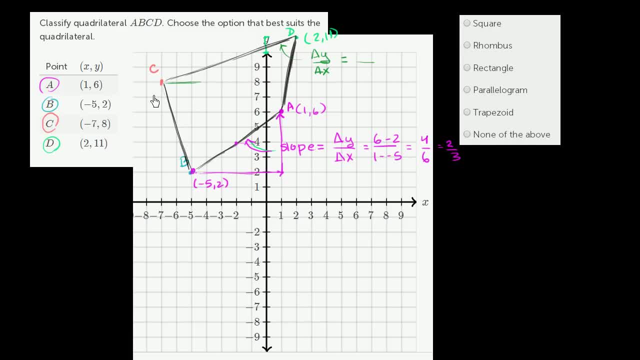 Our change in X: we go from. we're going from negative seven comma eight all the way to two comma 11.. So our change in X: we're going from negative seven to two, Or we could say two minus negative seven. So we go, we are increasing by nine. 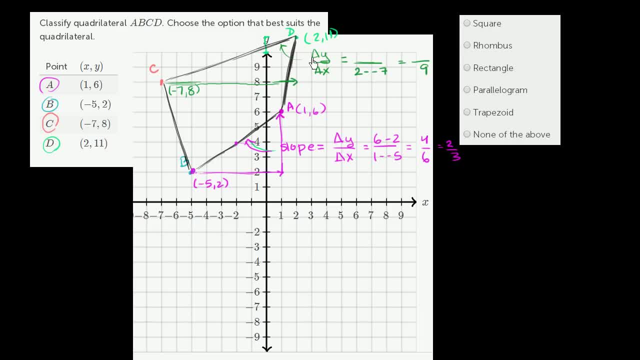 That's our change in X. So that's going to be equal to nine. And then our change in Y. well, it looks like we've gone up. We've gone from eight to 11. So we've gone up three, Or we could say 11 minus eight. 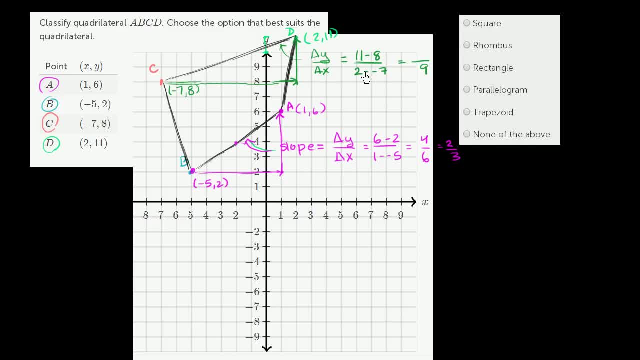 Notice: End point minus 12.. End point minus start point. End point minus start point. You have to do that on both, on the top and the bottom, Otherwise you're not going to actually be calculating your change in Y over change in X. 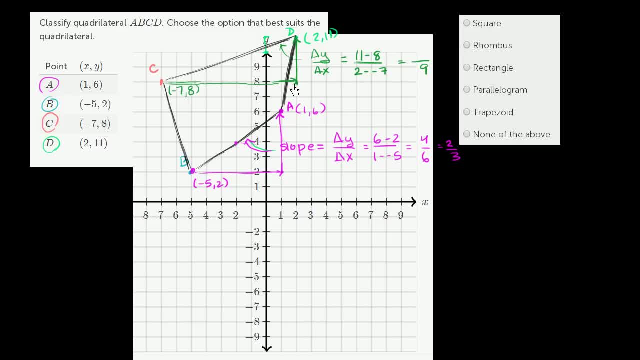 But you notice our change when we go. when our X increases by nine, our Y increased by three. So the slope here is equal to one third. So these actually have different slopes. So none of these lines are parallel to each other. 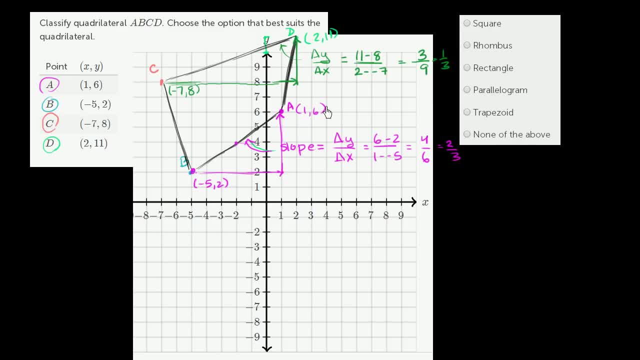 So this isn't even a parallelogram. This isn't even a trapezoid Parallelogram. you have to have two pairs of parallel sides. Trapezoid: you have to have two pairs of parallel sides. Trapezoid: you have to have one pair of parallel sides. 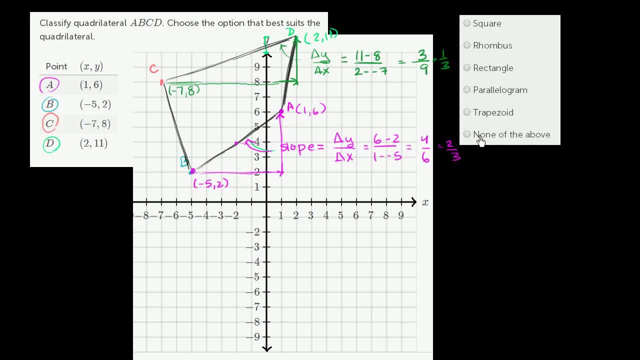 This isn't the case for any of these, Or none of these sides are parallel, So we would go with none of the above.